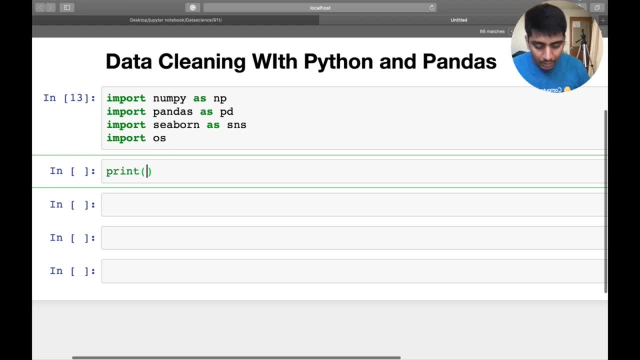 ESSI'm going to start school of code for this example here. I'm going to select all of these two, which ones will be available to you first, And I'm going to copy all the keys to theuffs in the office. So I was like I can see on your screen: Come over here I'm. 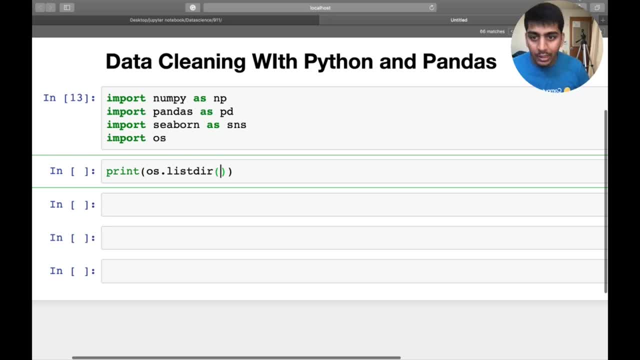 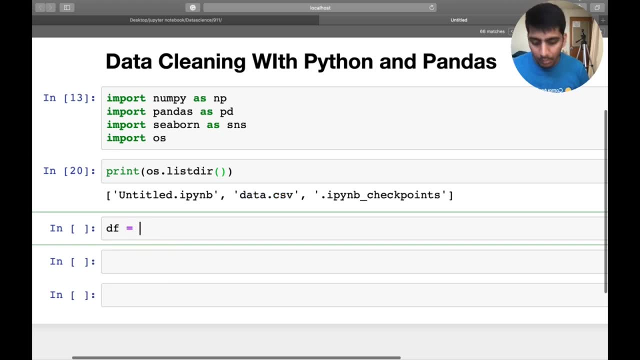 So the file is already there. So I'm going to say: list dirs. These are the files. here You can see the CSV file, So let me try to read it. So I'm going to say: now see the problem. So pdreadcsv. 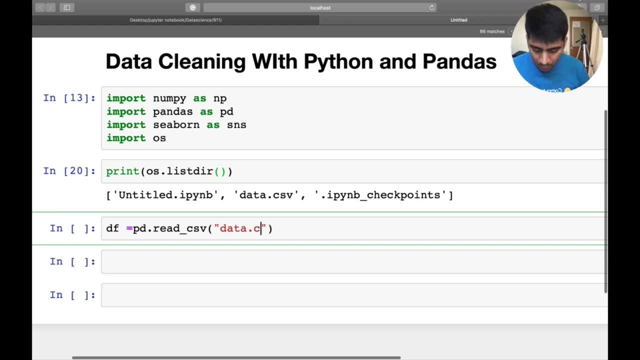 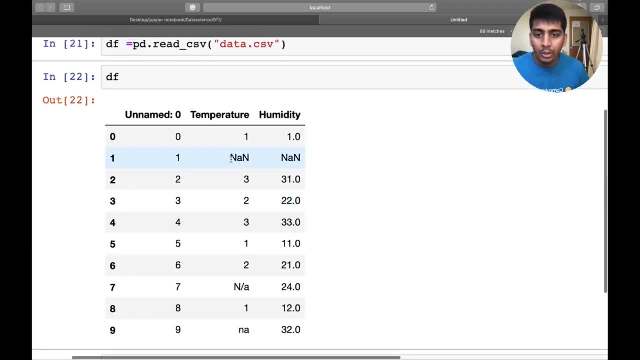 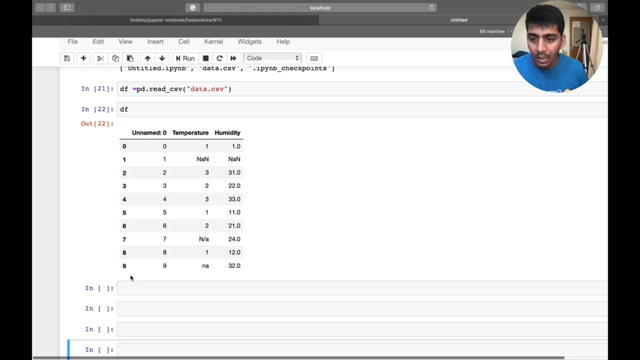 All right. So once that is done, I can say DF to essentially show you what's in the data set. So here you see, we have NAN value, We have NAN value right Now. we have NA value, N slash A value and we have NA value. That is this. Now, if you check now, see this what happens? Now this is the problem which most of the people are not aware about. So if I say DF, dot is null, now see what happens. 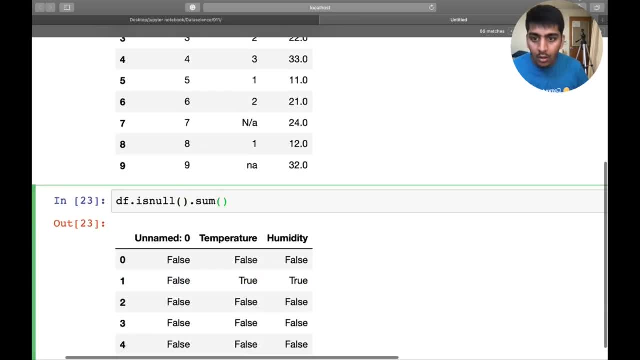 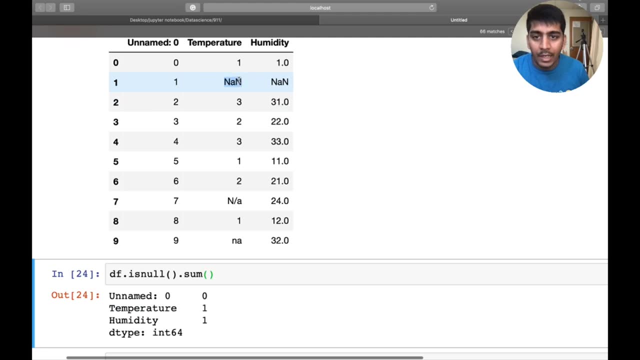 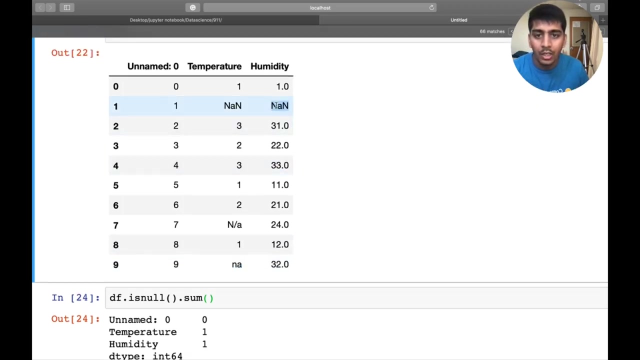 Okay, So essentially it's going to give me this. So it says temperature as one none value. Now, what about this guy? See this: We have one NAN value. What about this? It did not count these value, So pandas was not able to recognize these as none values. Now, how do we handle this situation? It's pretty important, right, Whenever you're doing any kind of analysis. So, similarly, here we have just one, So that's fine. So the way to tackle this problem is to 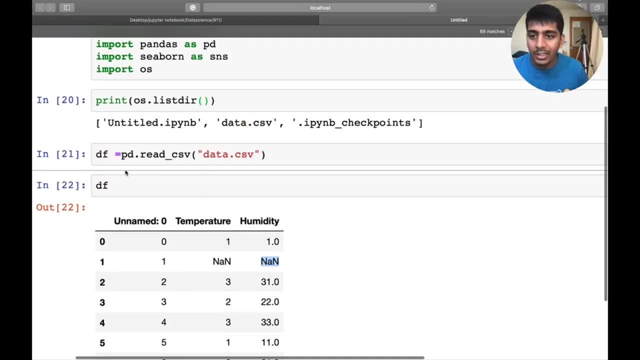 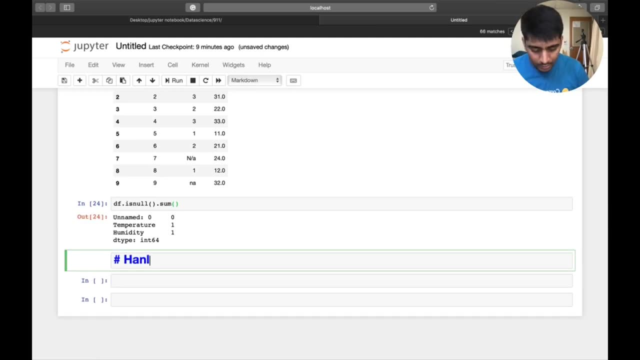 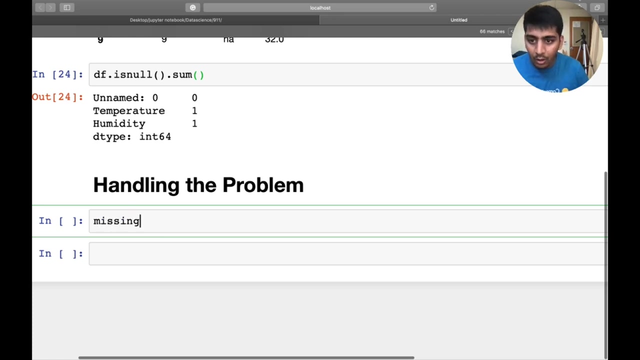 in pandas would be. So, while reading the CSV, you should define: Now, this is the problem, right? So now let's say handling the problem. Oops, sorry for the spelling mistake. All right, So handling the problem. So now, what we will do, guys, is basically create a list of missing value So it can be NA. 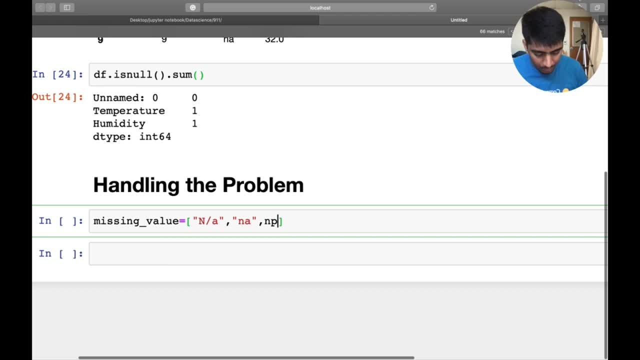 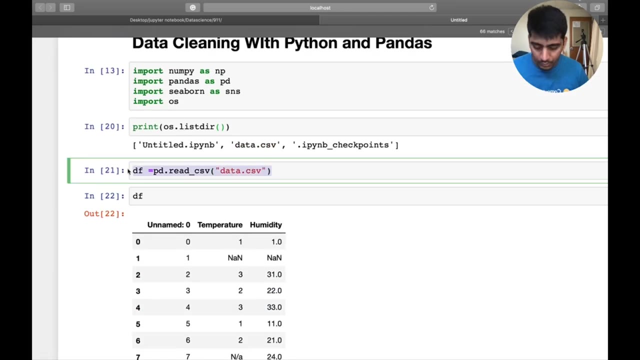 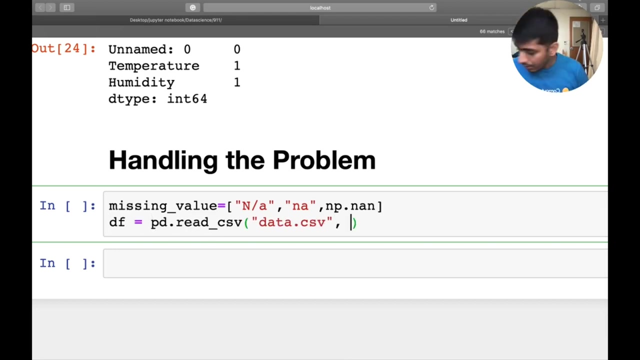 It can be NA, It can be NP, dot, NAN, right, So these are essentially all the types of missing value that I am expecting right now, Right now, while reading the CSV file. let me just show you the art of doing this. So, missing values Now: if I say PD, dot, read CSV. And if I say, if I pass in an argument known as NA, underscore value. 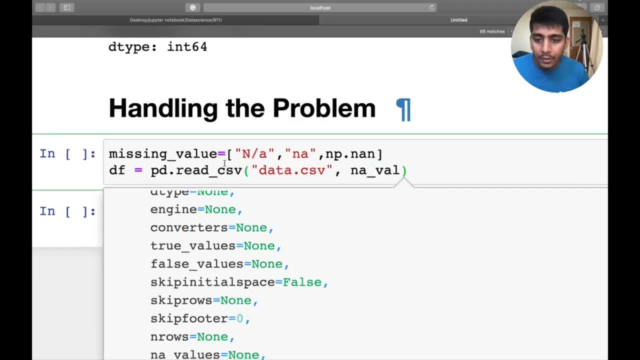 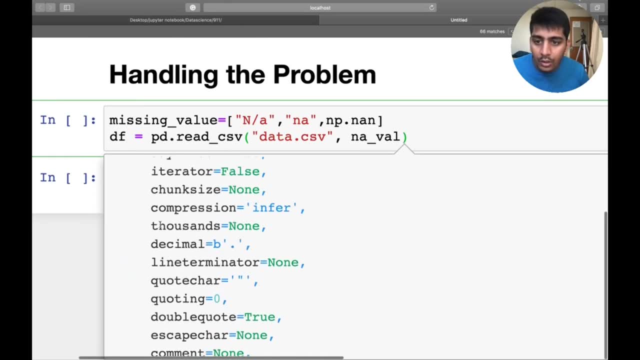 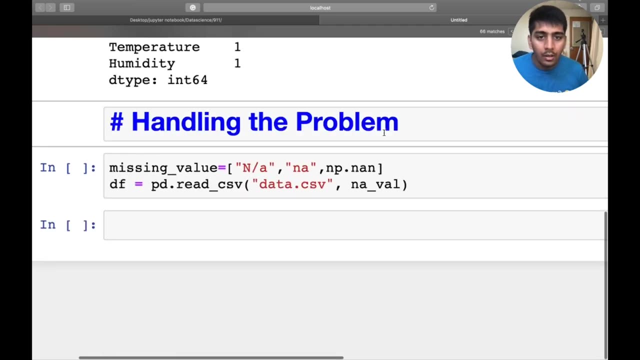 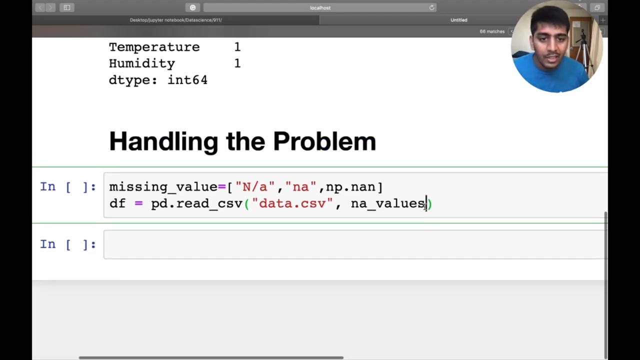 So if you do shift tab right And if you essentially just scroll down till you see this function known as NA underscore values, So it should be there in somewhere NA Here you see. So NA underscore values by default it's none, So we will do this. Let me just run this. So we are going to say NA underscore values and we want to supply our custom NA values, So we will say missing value, right? 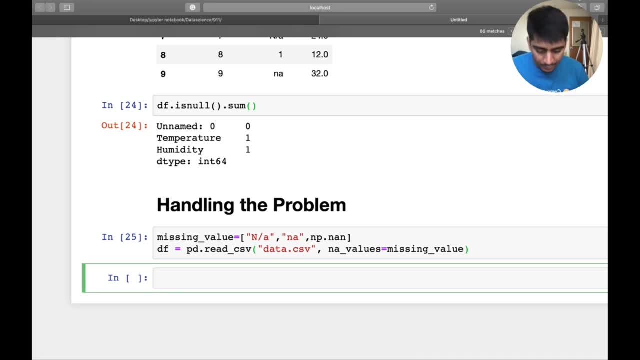 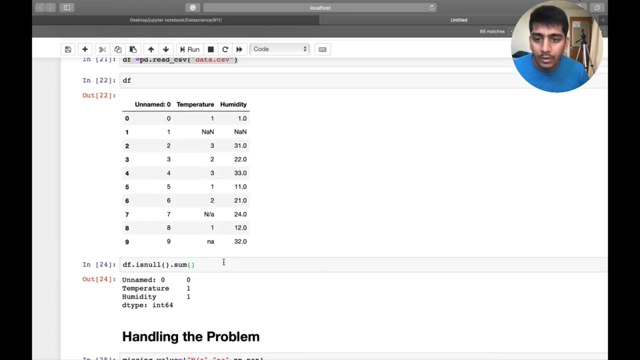 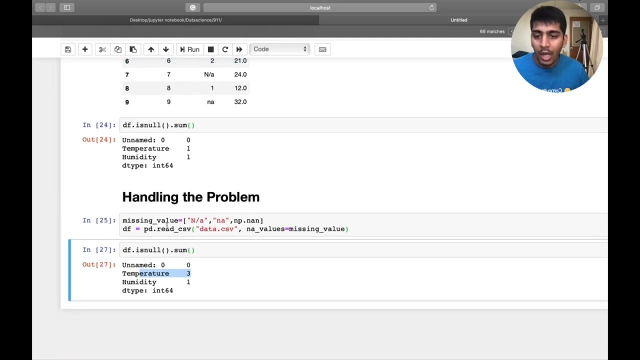 So now, if I run this and if I say DF, dot, and if I say is null right, And if I do some, So here you see, now we are able to recognize all the three NA values. So essentially, this one, this one and this one. So, if you're so, this is very important, So you learn something new. to tackle NA values, We are using these methods, right. 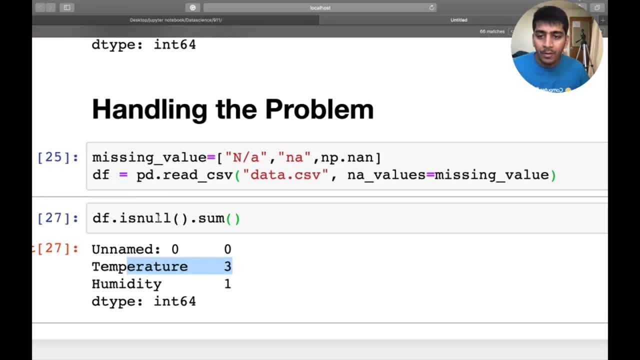 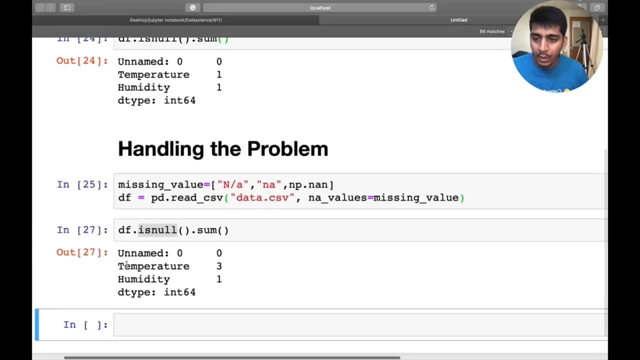 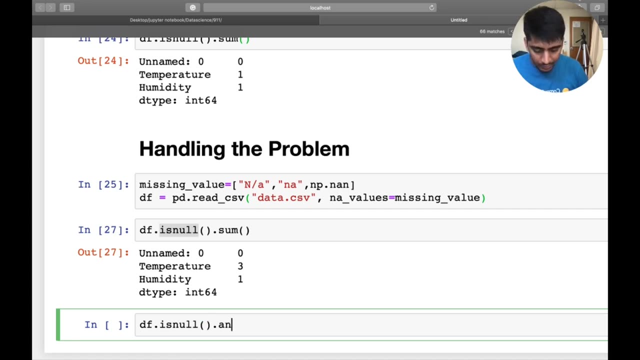 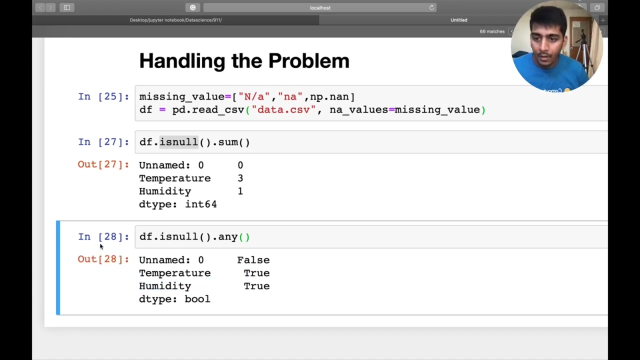 Now how can you check whether the, whether you have any empty values, So simple, we can say is null And you can just calculate the sum on that. Another method you can do is DF, dot is we can say is null And we can say any. So this will basically check. So here you see, we have true, that means we have some NA values. So now we can also visualize those NA values, So we can essentially plot the heat map. 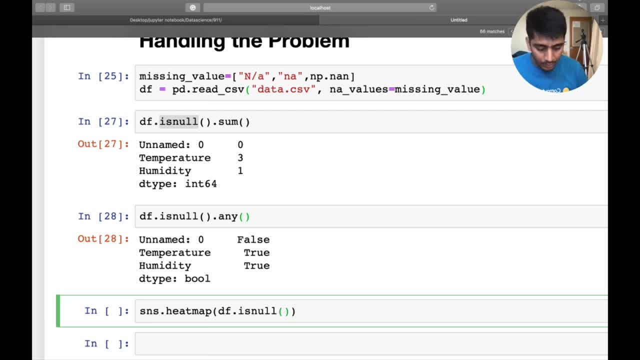 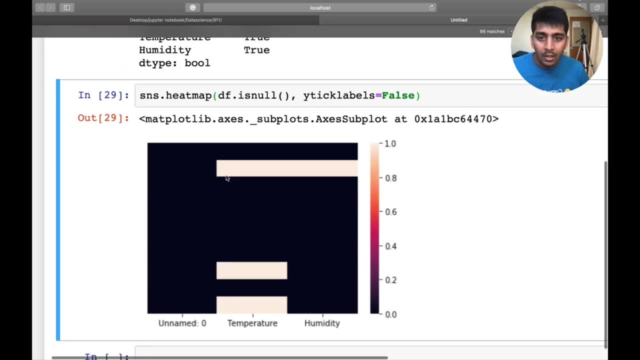 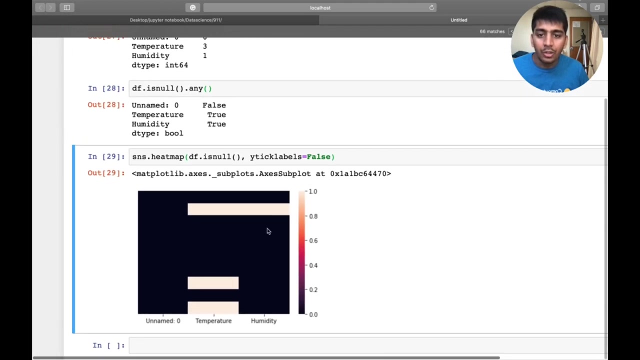 So I can say DF dot is null, Right. Essentially, this is going to give me my Boolean values And I'm going to say false. So here you see I have. this color indicates, if it was totally black, that means the data set is perfect. But now, right now, since we have in temperature, you can see we have three of them. So we have three non values. Similarly, the humidity: we have one. So this shows that we have one, one NA value. So I can say a not. 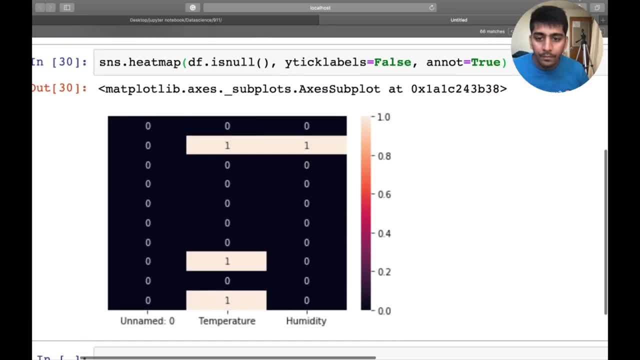 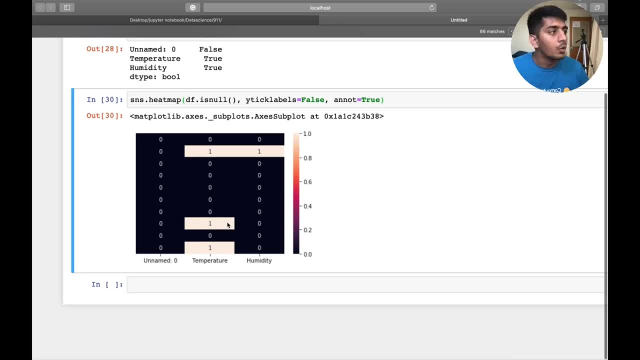 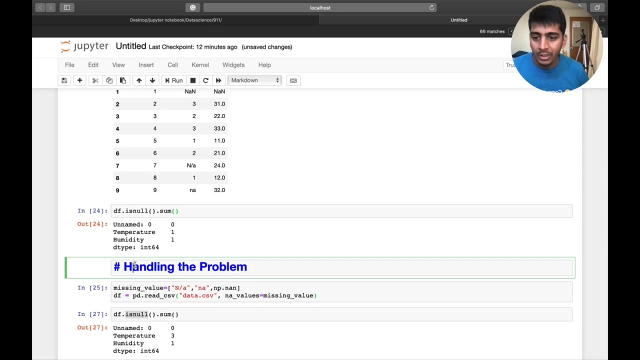 True. So here you can see. essentially, this is where we have the NA values, where it's also showing us. So this is a pretty good way to visualize your data set using pandas. Just give me one sec. So we learned about detecting the NA values, right? So this was the art of detecting the NA values, So let me just write step one. 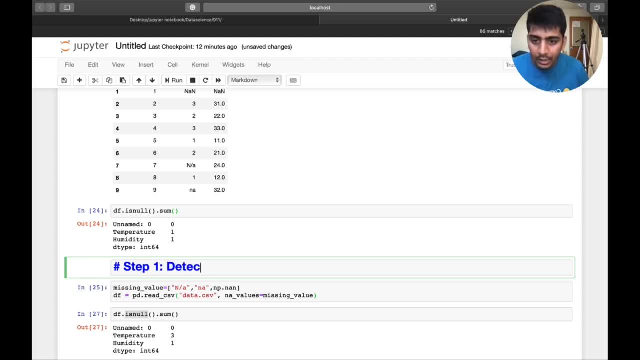 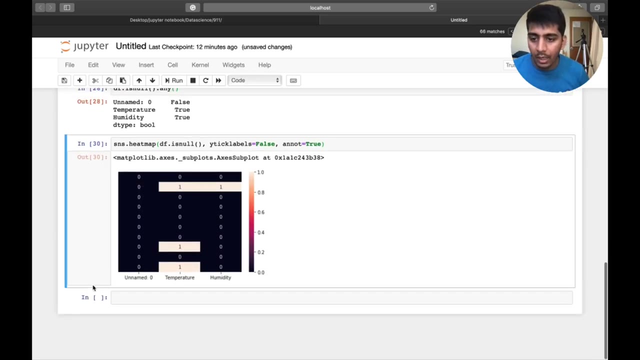 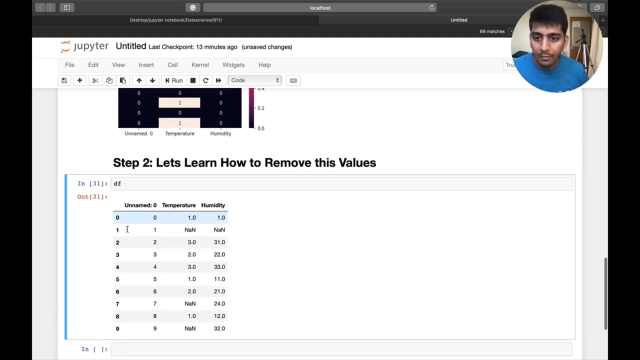 detecting the EEC, detecting and then and slash eight and n values. We learned about this. right now, we will learn how to remove these values. So, all right, so we will learn how to remove all of these value. so, essentially, i want to show you the data frame. right, this is what we had. now, um, let me just quickly open my snippets, right? 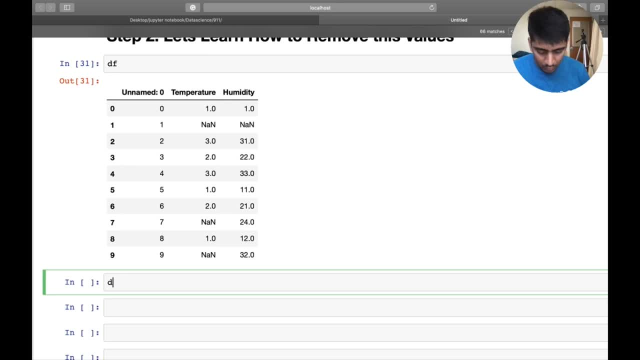 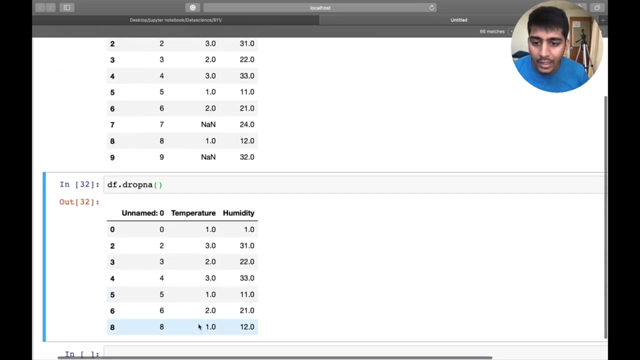 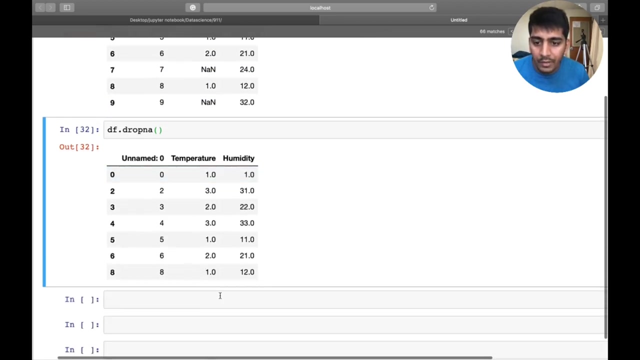 and hopefully, if this makes sense, so you df dot, i'm gonna say drop, and if i say drop, na right. so if i just do this, uh, let's see what happens. so, essentially, if you observe all the na values, even this one, now we are taking care of this one, this one and this one, all of these, uh, we actually 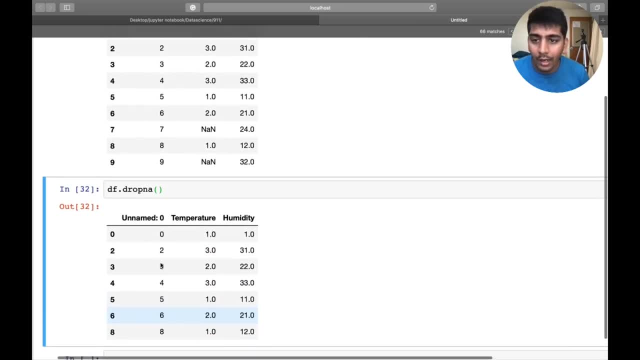 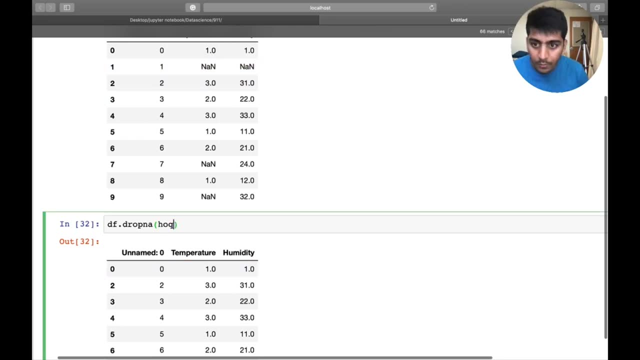 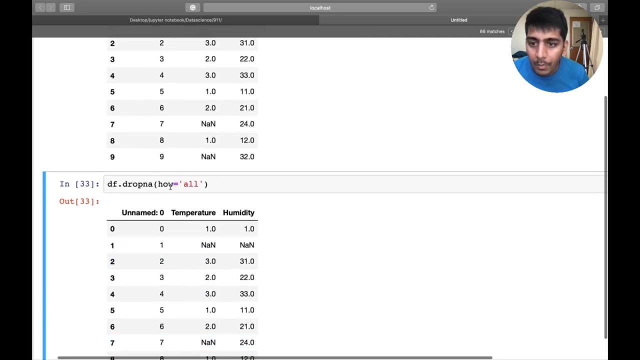 drop all of them, right. but let's say we don't want to do that, right. we only want to drop where the entire row is none. so simply we can say how? equals to how, equals to all. now, if we do that, so, oops, drop any. let me quickly open my snippets as well. so drop any, and how. 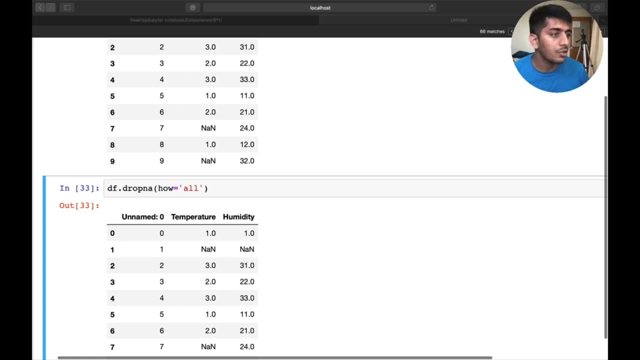 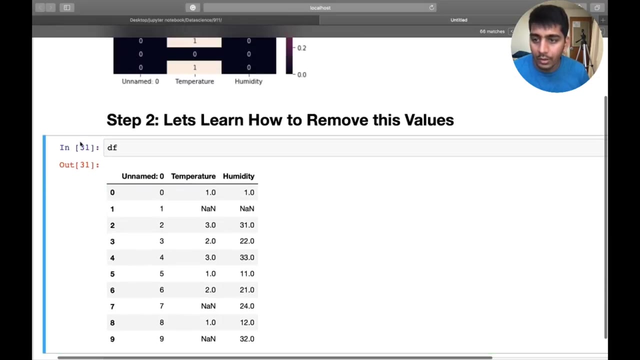 equals to all right. so let me just copy a small piece of code to make this concept better, I mean to make it better, to explain it to you in an easy way and not in a complicated way, right? so essentially, what I will do is I'm gonna. 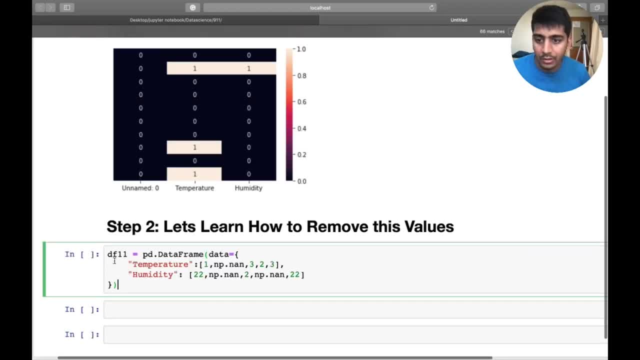 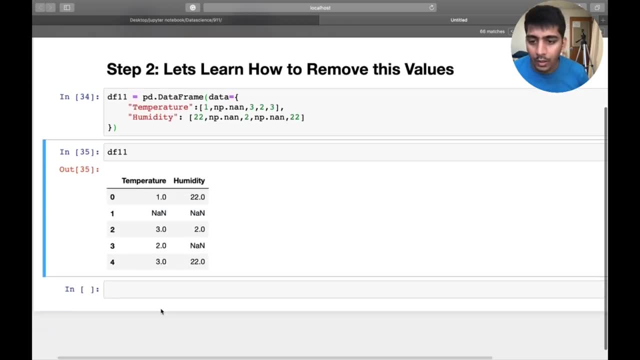 remove these and let me just paste this data frame for now, just for explanation. so if I say df, dot, 1, 1, so we have this data frame right since, excuse me. so here you can see, we have one- none values here, and we have second- none values here. 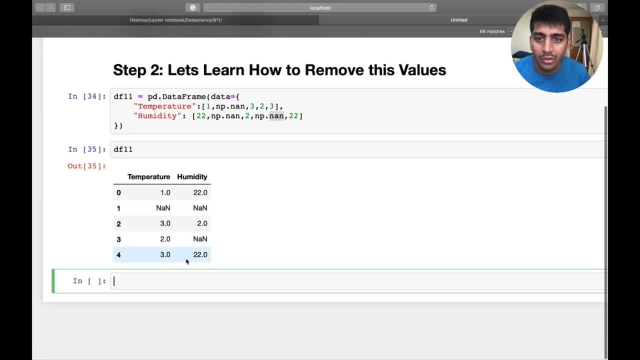 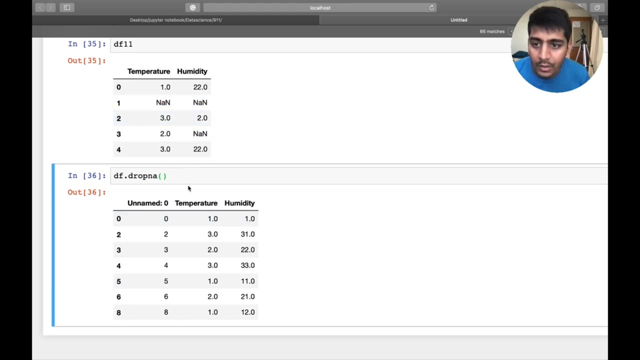 right, essentially just a small data set to to demonstrate what's happening. so now in on this data set. if I say, guys, df, dot, drop any and let's run it and see what happens, so we will compare both of them. so we had this, any values right? so it it dropped that row. 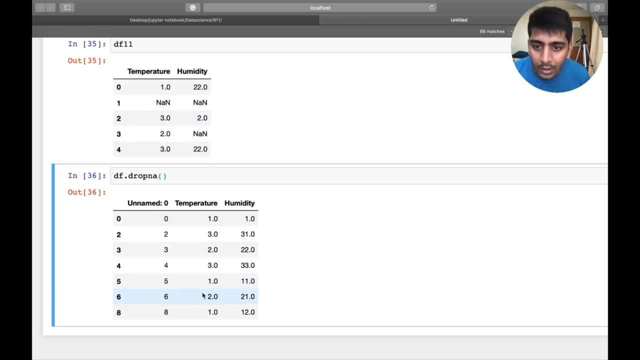 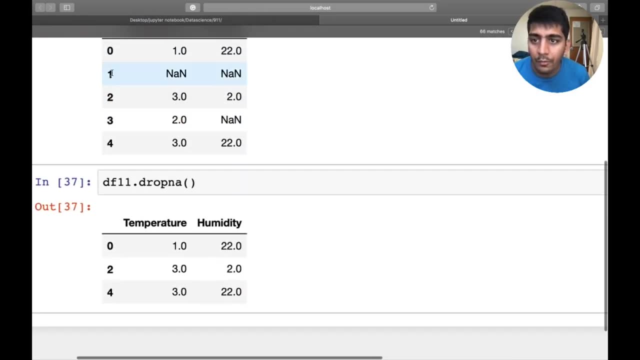 completely. we had this one, so it also dropped that row. oops, I have to say df 1: 1. sorry, really sorry for that confusion. so essentially now, if you observe, this entire row was dropped and even this row which has just one values was dropped. but I don't want to do that. I want to say when. 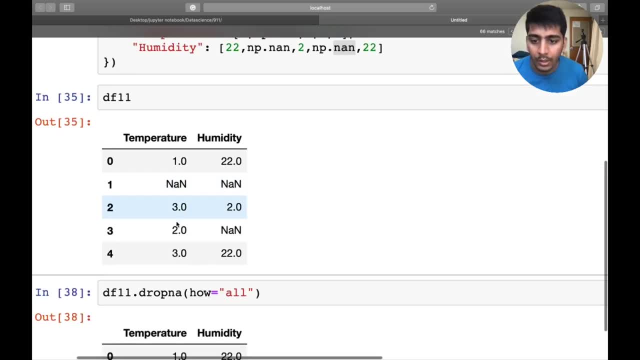 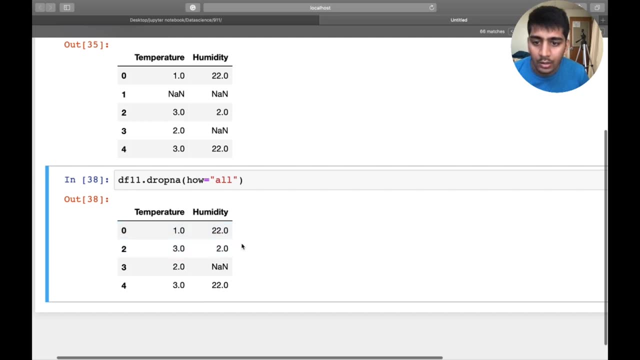 there are all, all the rows are empty, then only do it. so if I essentially just say: how equals to all. so now you can see, here both the values are none, right, so it's removed, and here only one value is none, so it's not removed, so you can just. 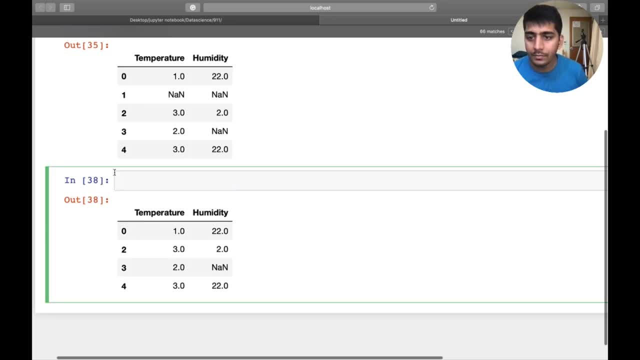 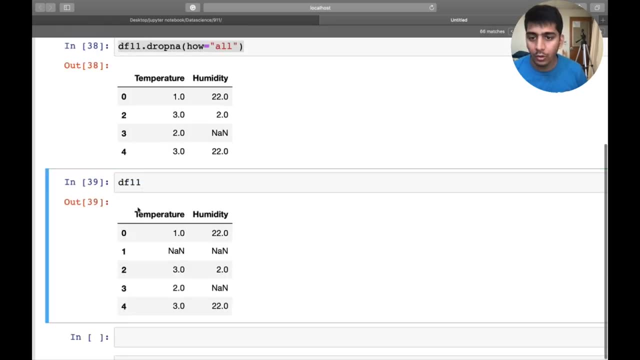 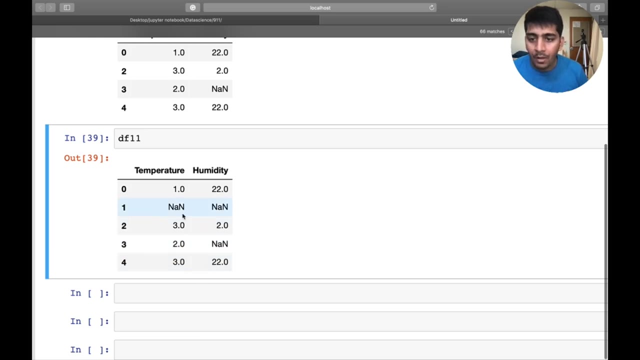 specify how equals to none, right? so essentially, I'm gonna keep this. now let me show you the art of filling data. so so, this is a data set, right? so the first method that I will show you guys would be filling it with all zeros and then manipulating it. df, dot 11, fill in a and I want to fill with 0. so now, 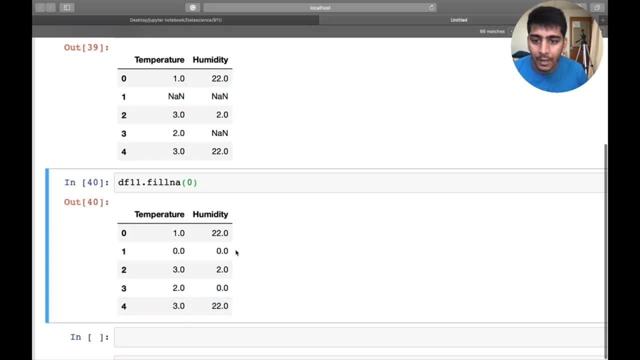 let's observe what happens. so here you see. we had any and any, so we have zeros and essentially 0 over here as well. but when you're doing data analysis, this is not a good way to write zeros. we don't want to do that. we have, we want some. 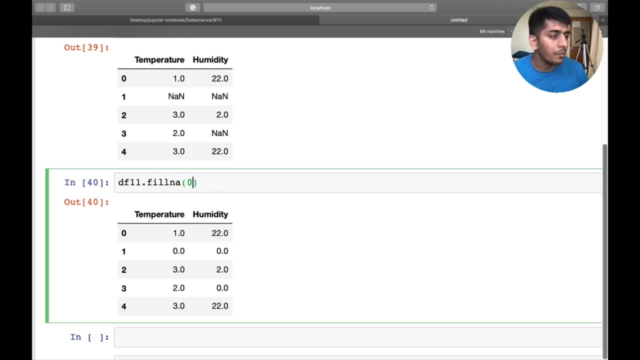 kind of method to you know, we don't want to do that. we want some kind of method to you know, get, write some kind of data there. so let me show you a method of FF field, this forward fill and backwards fill. so let me just quickly, for just one second, let 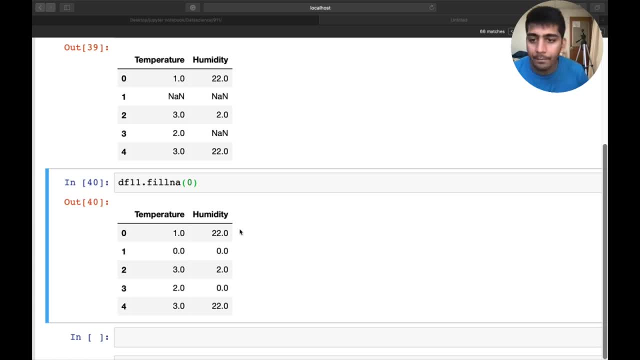 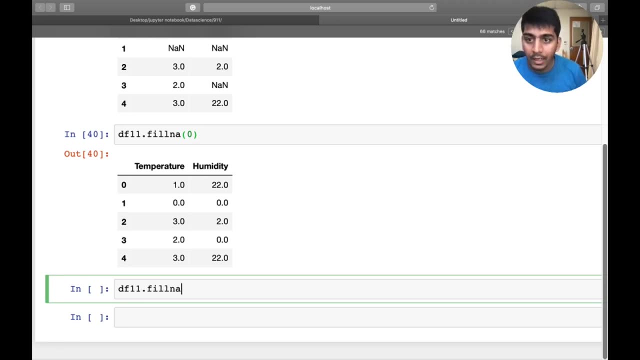 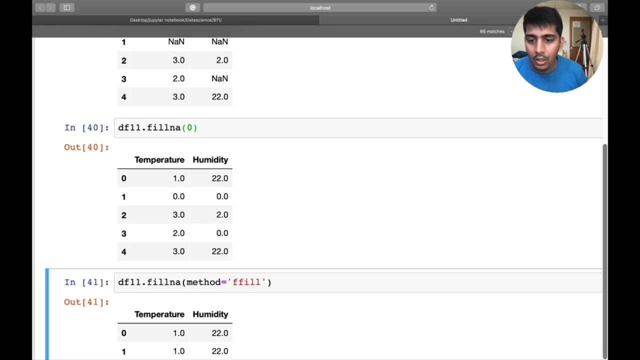 me just go to my snippets right so I can show you that. so this is what it did. right now let me show you the df 1: 1 dot fill in a right and now, if I run the method, equals to FF forward fill and so observe what happens now. so, but before that one, I just print my data. 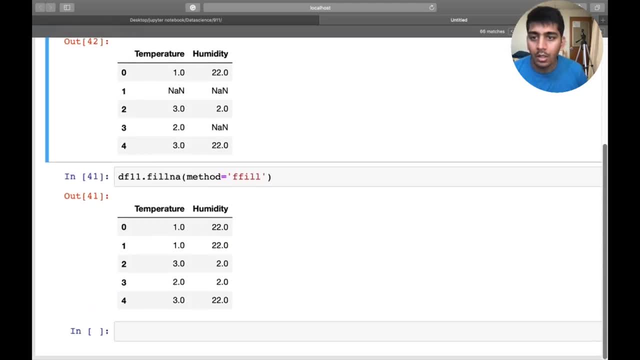 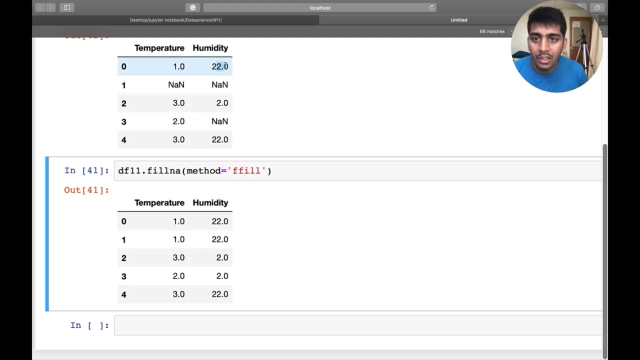 frame also, so we can compare both of them simultaneously. so let's observe what happened. so here we had nothing, so this one got copied here, right. so this one got copied here. this: we have 22, so 22 got copied here, right. and similarly, we had nothing here. so the upper value is 2, so the 2 got copied here. what? 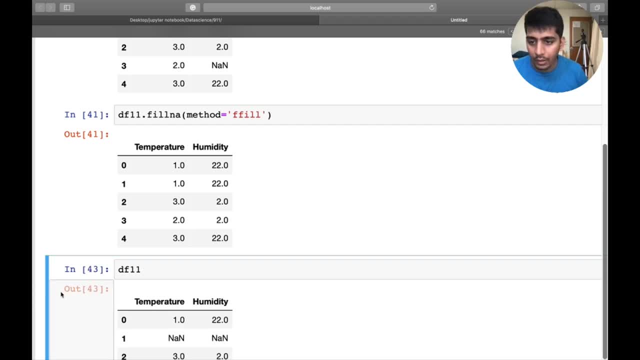 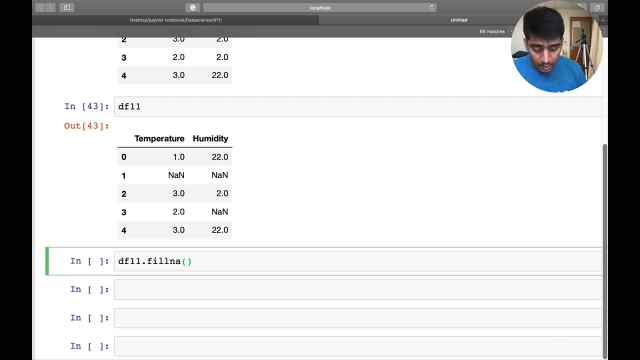 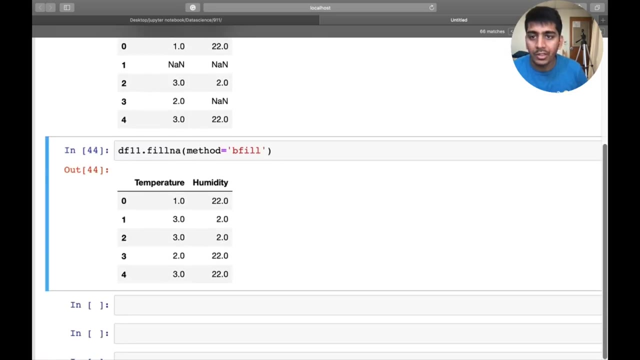 happens if we do the backward fill. so let me essentially demonstrate that as well. so I'm gonna say fill in a and I can set supply, a method, and I can say backfill, so let's see what happens. so essentially, these are my columns right now. this 3: 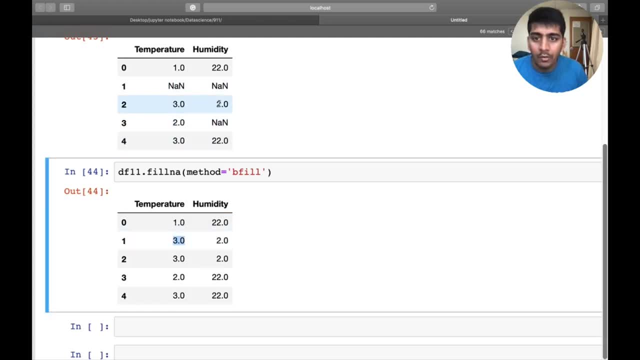 would be copied here. this is backfill here. you can see we had 2 here, so 2 is copied here, and essentially we had 22, so 22 got copied here. you can see this is not a good way, guys, to do this, but there is one more way, which is just. 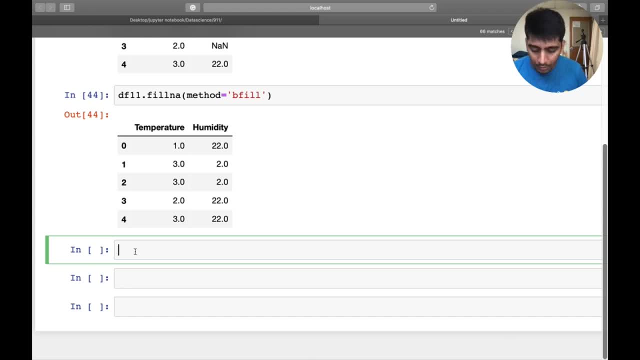 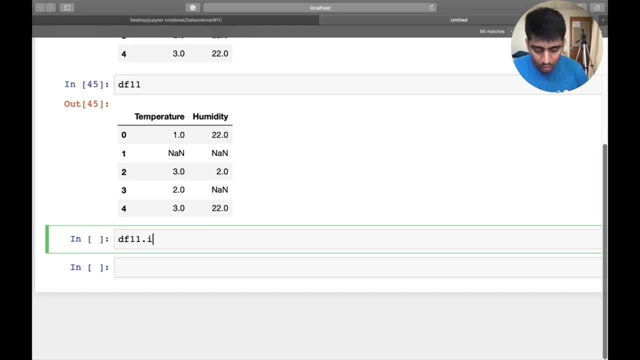 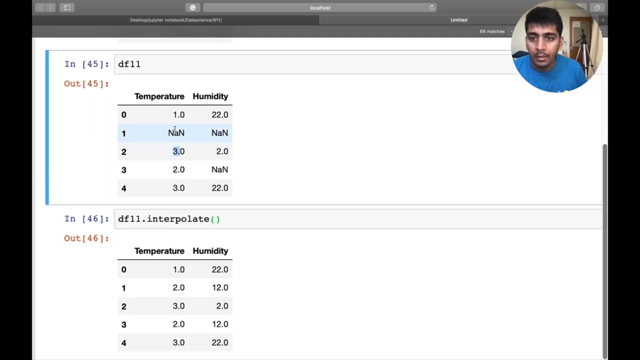 called interpolation, right? we also want to do interpolation on the data set. so df dot 1, 1. let me just print that so I can say df dot 1, 1 dot. interpolate, right. if I say that? see what happens now. let me explain you. so 3 plus 1 is 4 divided. 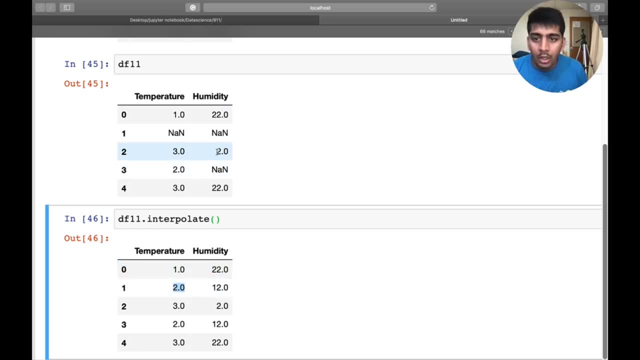 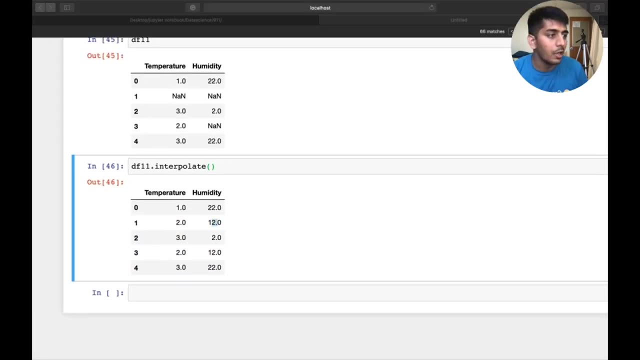 by 2 is 2. so we have to. this is interpolation: 22 plus 2 is 24, divided by 2 is 12. so we have 12 value 12 here. so here you can see. this is the art of in interpolation. alright, so essentially we learned about that as well. now, 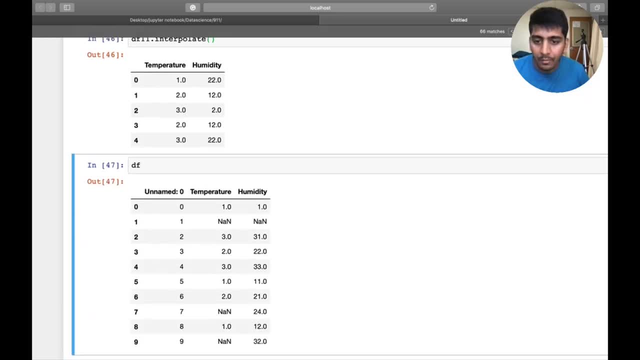 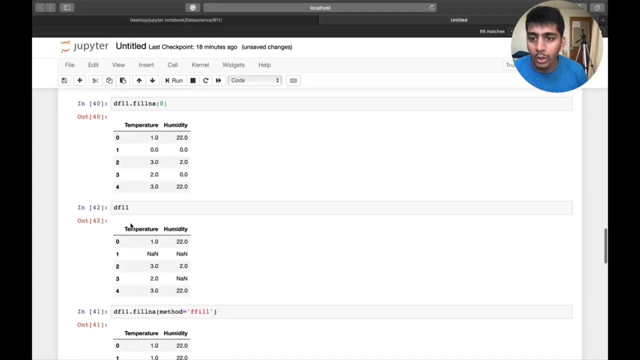 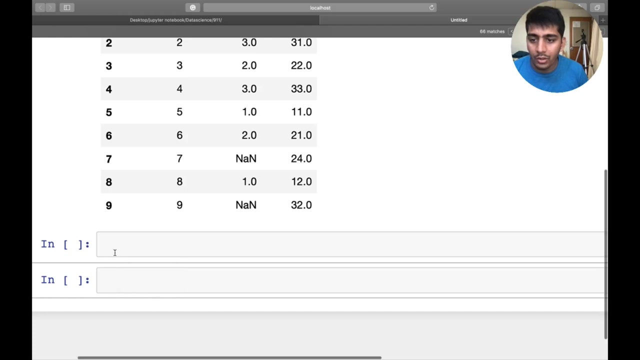 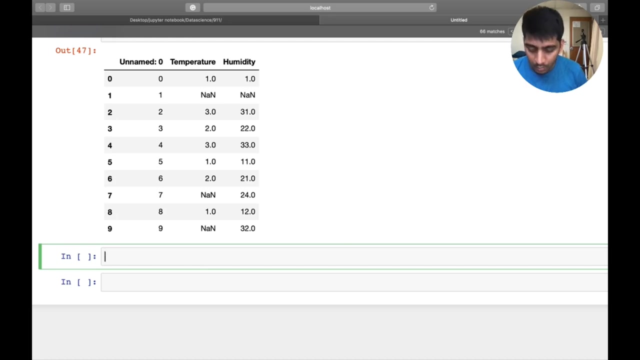 essentially, let's go to the original data frame, which had all the none values here, right? so so you can use any of these methods to do your cleaning on on your data set. so we learn how to do all of these, right, so let me just quickly, just drop all of them. so df, dot, or let's say df. 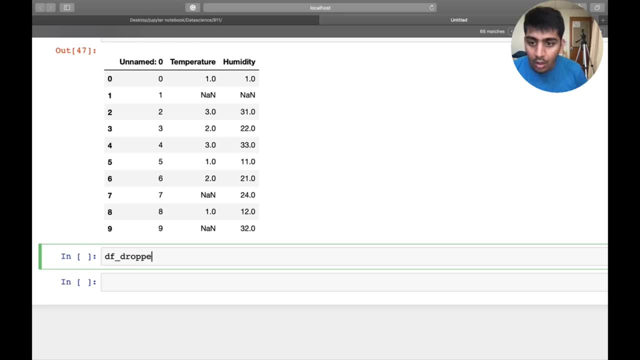 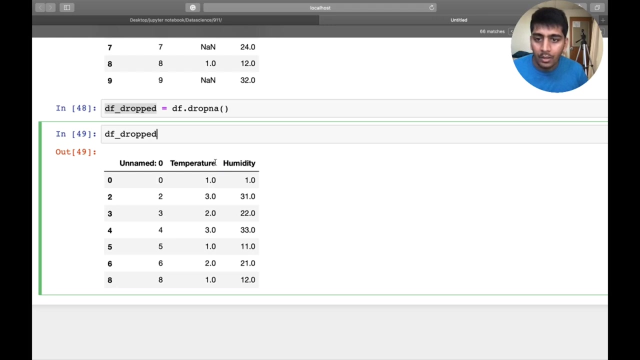 underscore dropped is equal to df dot drop. drop any right and just run it so you can essentially see the output. so now you can see we have removed all the rows and column that was dropped right. so, as I said, it's not a good method to do. 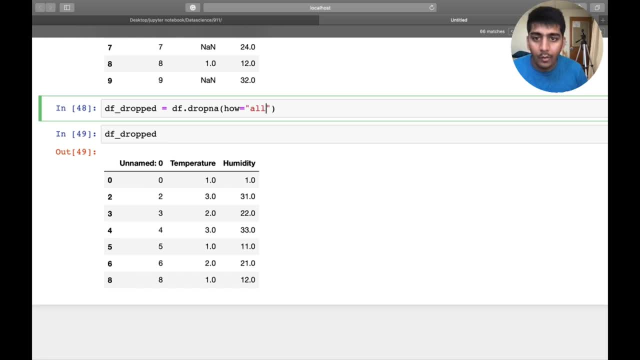 this. if you want to do this, you can supply again our. we can supply again our. we can supply again our. we can supply again our equals to all. so it will only remove the rows and column that has both the none. equals to all. so it will only remove the rows and column that has both the none. 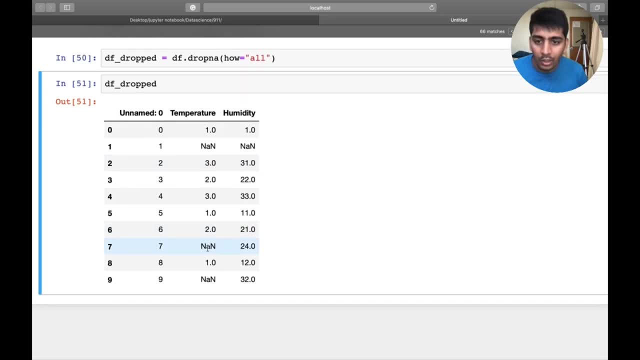 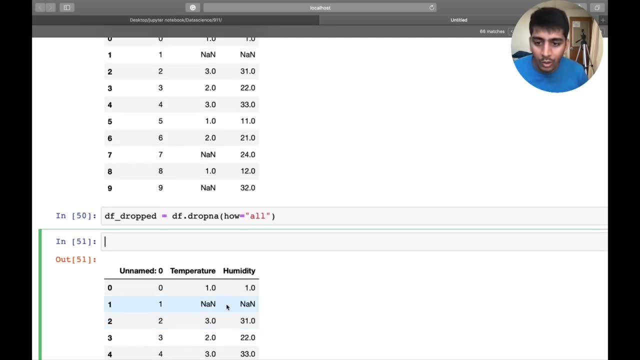 values. so essentially here you can see, this only had single, none values, so I did not remove it. so this is what it did. so this was not removed. you will ask me, hey, why this was not removed? because here we also have a value unnamed, zero. so if all of them are zero, then this would remove it, so we can just say df. 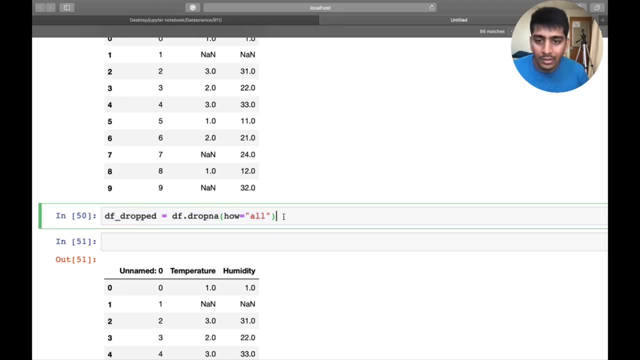 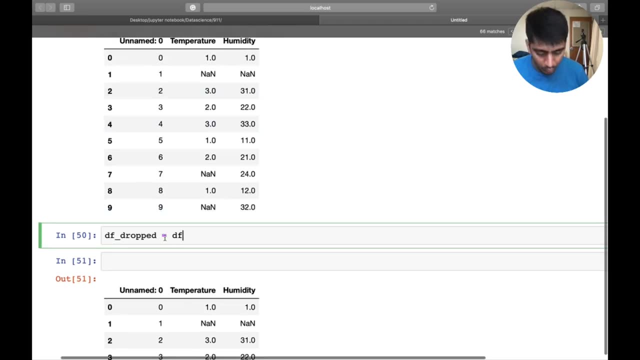 dot n a, or instead we can just use a method known as interpolation right dot n a, or instead we can just use a method known as interpolation right. so this is my data set right. this is how it looks like, so I can say interpolate. so this is my data set right. this is how it looks like, so I can say interpolate. 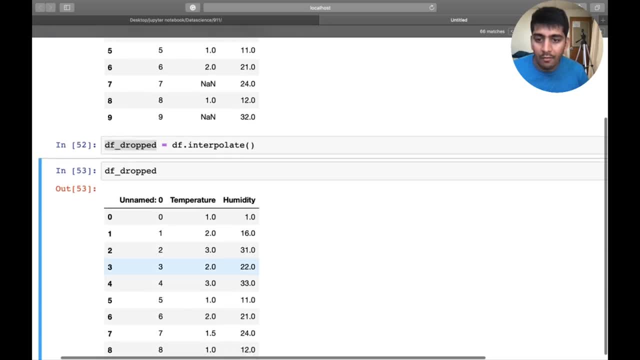 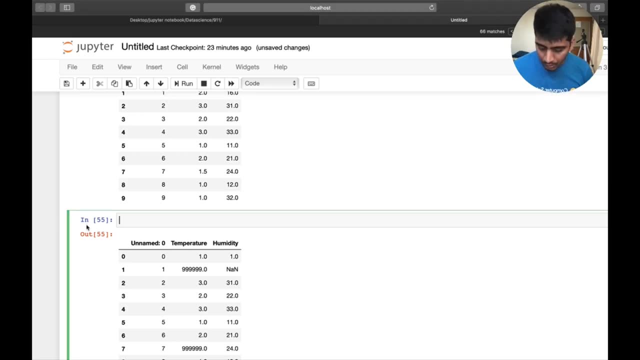 and now, if I print it, so we have values now. so that's it for this. one more thing that I forgot to mention is, basically, if you want to substitute the values, right, so let me just show you what I mean by that. so here I have the data frame, right. 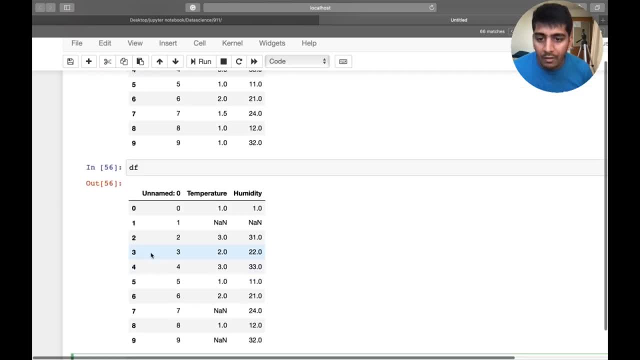 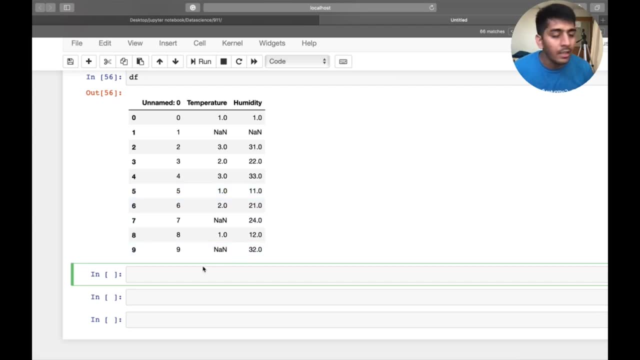 so let me just print a small data frame. so I have a data frame with. do you agree? now, instead of n, a and I want to substitute, let's say, or. instead of 0 or 3, I want to substitute 99999 or any values or anything. right? so the way you. 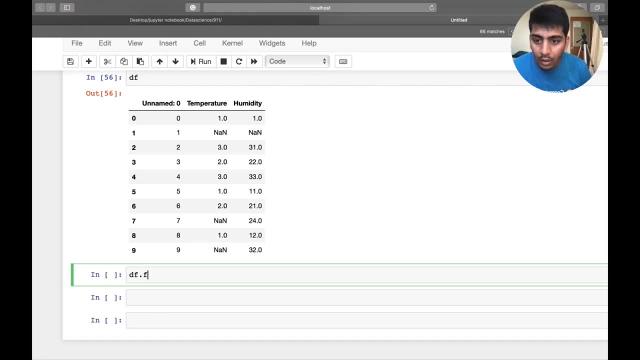 can do, that is, you can say df, dot. first of all you need a method known as fill n a. so so, which will take a dictionary right, and I want to fill all the temperature values where it says none, and I'm gonna make it do some reason. I. 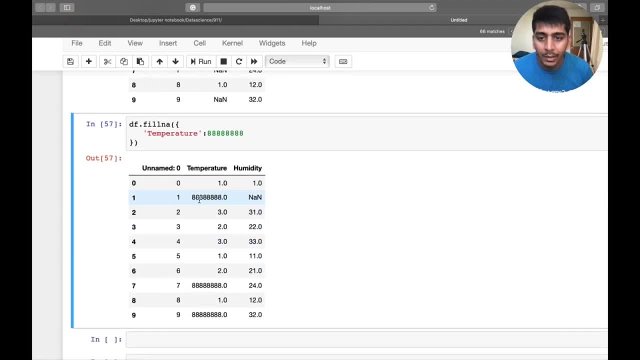 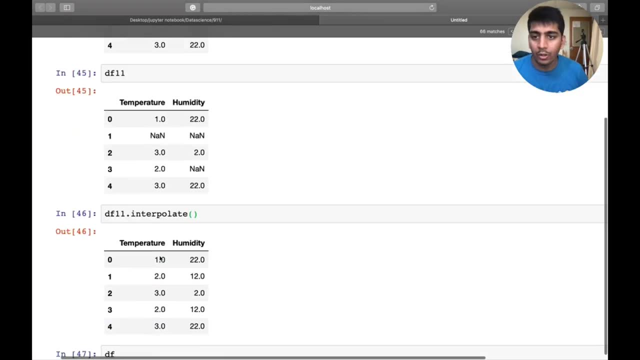 don't know, so here you can see. wherever it was n a- now it's a- did it, so you can also do this. just wanted to show you. so thank you for watching and hope you have enjoyed it. I also hope you have enjoyed this tutorial on data cleaning with. 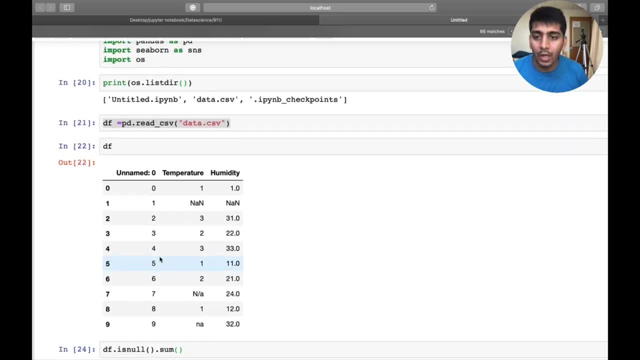 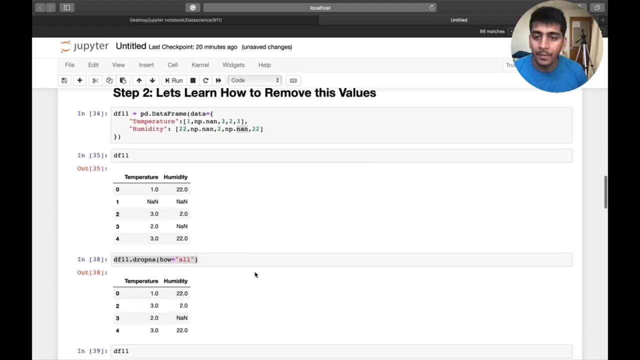 pandas and Python. if you have any questions or if you have any suggestions, do let me know by doing that in the comment section below, and I would be very happy to answer all of that. so, essentially, this was a new method that I taught you to visualize the data set, and then I'm going to show you how to do it. 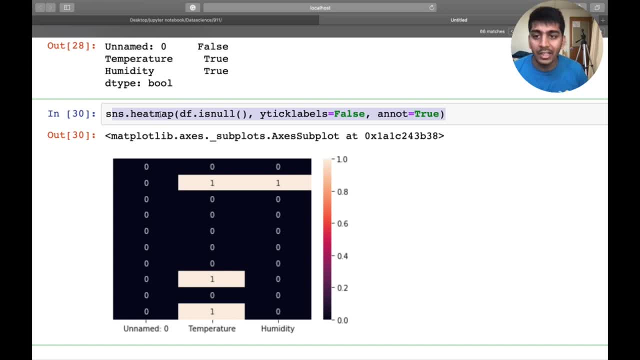 in a little bit later. so thank you for watching and see you guys in the next video.